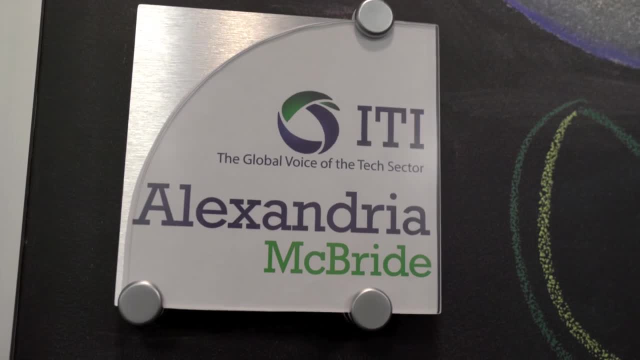 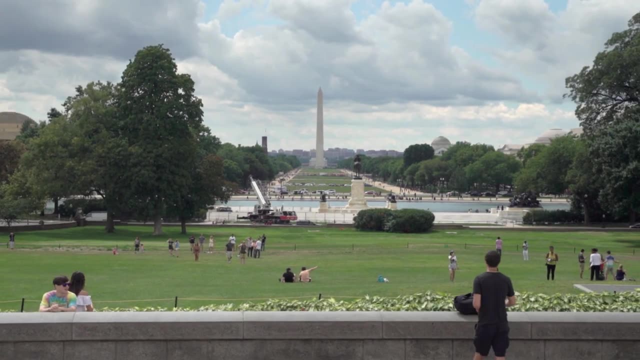 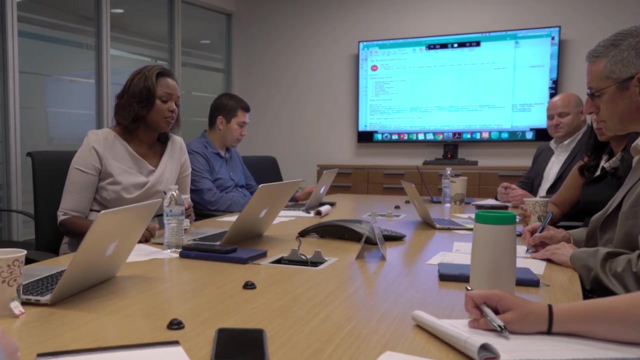 the Director of Environment and Sustainability at ITI. ITI stands for Information Technology Industry Council and we're a global tech trade association based in Washington DC. I work with technology companies and try to figure out ways that we can work with governments to come up with policies that work- policies that help the environment, but also policies. 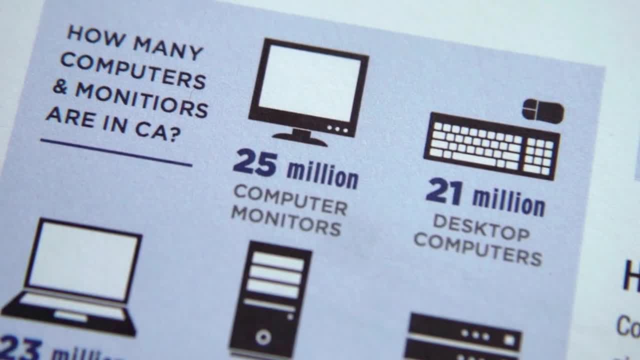 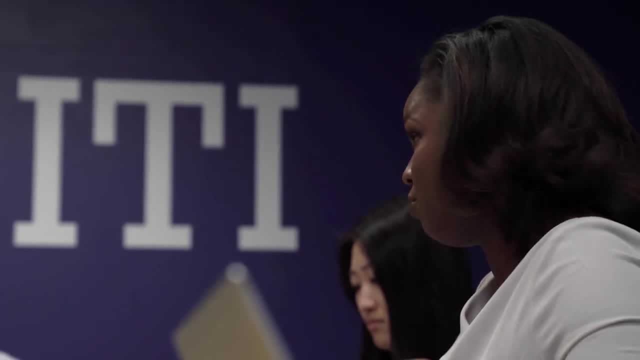 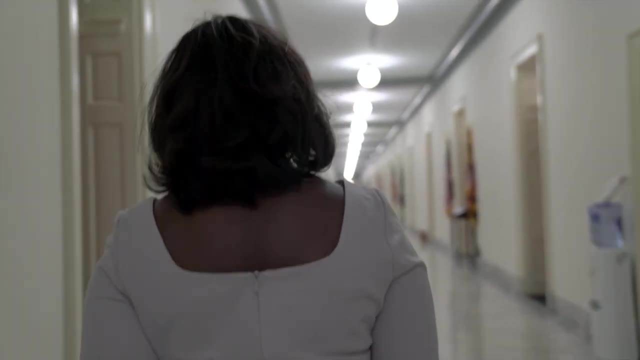 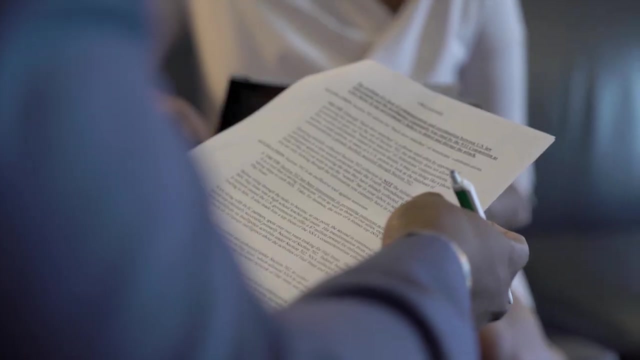 that make our companies continue to innovate, And what's exciting is the work that these companies are doing are very closely related to environment, sustainability and the types of changes we need to see. I'm able to go to different congressmen with really clear solutions and kind of say like hey, how can we come up with smart policies that allow? 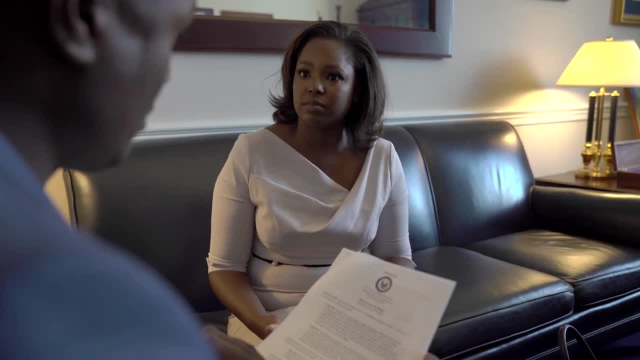 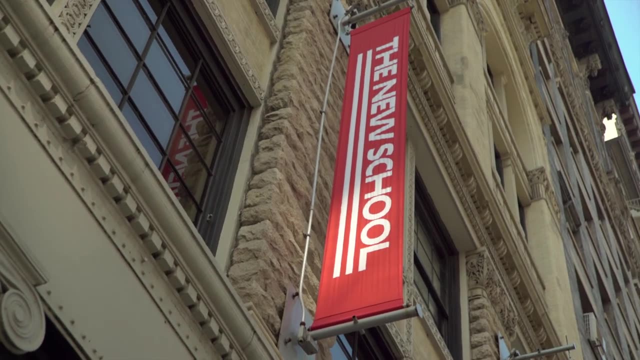 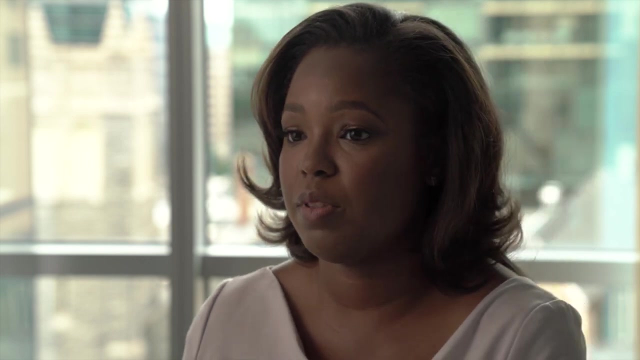 our companies to continue coming up with those solutions. I received my degree in Environment and Sustainability Management from the Milano School of International Affairs, Management and Urban Policy- IE- the policy side, or IE maybe with more science or maybe with a more social justice. 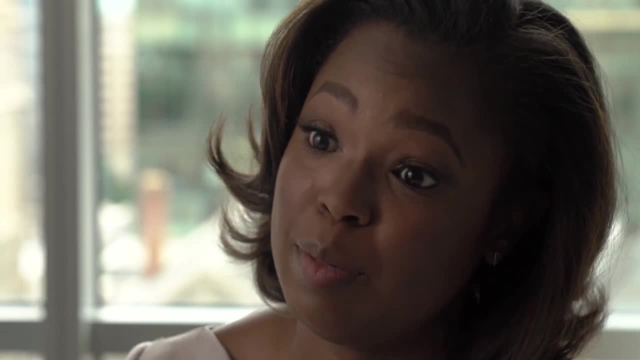 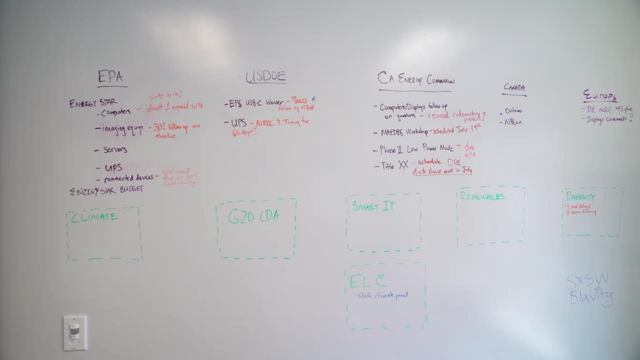 angle, And the benefit of my program is that I was able to get a sample of each. The new school helped me develop my passion for environmental justice by giving me a chance to study it and examine it in a way that I had not done before. I walked away with an experience that 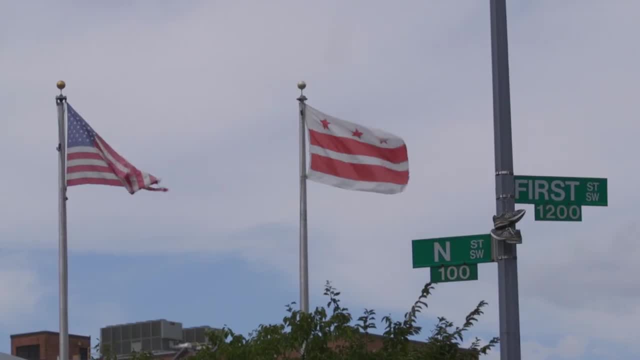 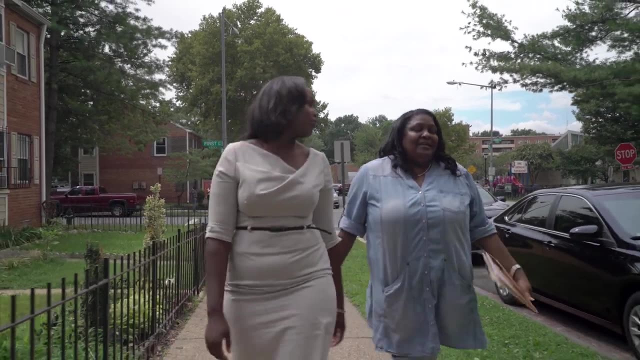 was valuable to my work here at ITI, as well as to the work that I do in the community. I also now chair the Environmental Justice and Sustainability Council. I also now chair the Environmental Justice and Sustainability Council. I also now chair the Environmental Justice and Climate Committee for NAACP DC Chapter And that means I work on issues. 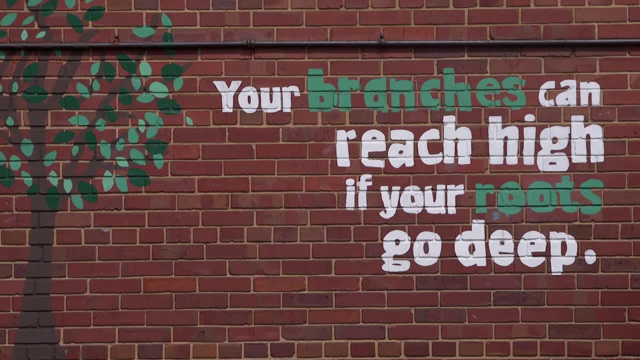 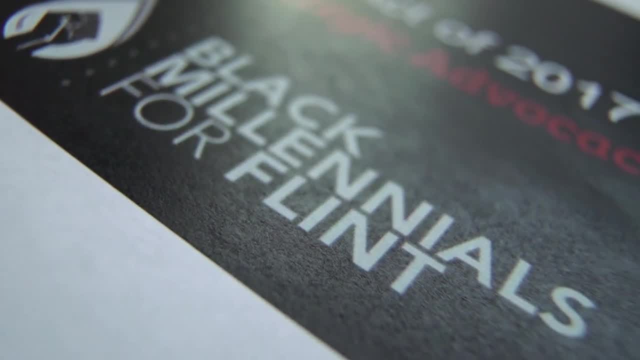 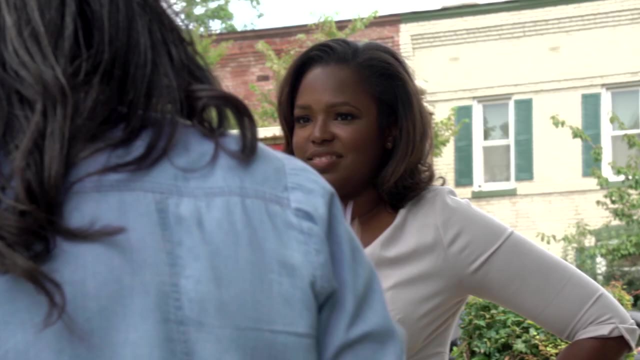 affecting the DC community around environment and climate justice. One thing I've learned at the new school was how to enter a space respectfully. I got to know other organizations that were on the front lines, that were in the communities that were being affected worst or hit the hardest. We are working together to convene and share best practices and advocate. 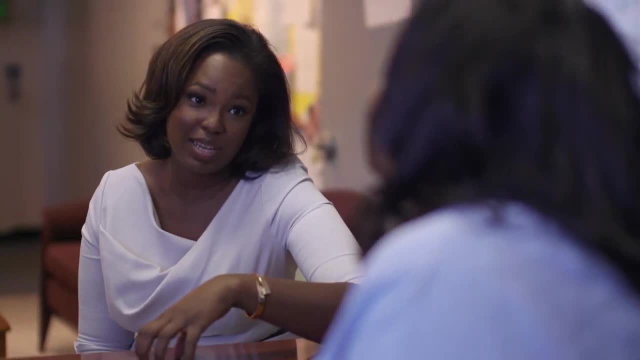 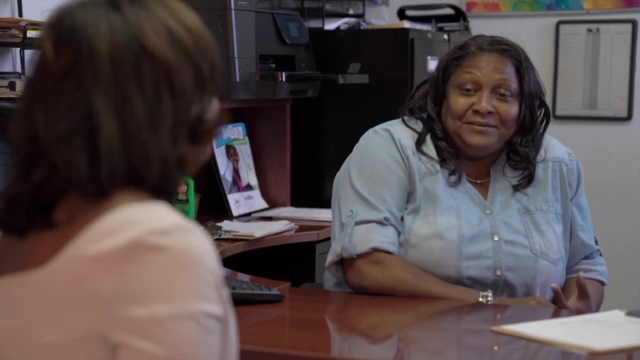 as a community group. We took some time to partner on Earth Day back in April. There's so many people. We had a lot of people out there. Yes, we had folks from the mayor's office, we had our resident manager and the DC Housing Authority behind us. DC. Empowerment. A lot of folks came out that Saturday in all that rain. I love the city and being able to fight for and advocate for the people in the city helps me come to work every morning and feel good I'm able to take the